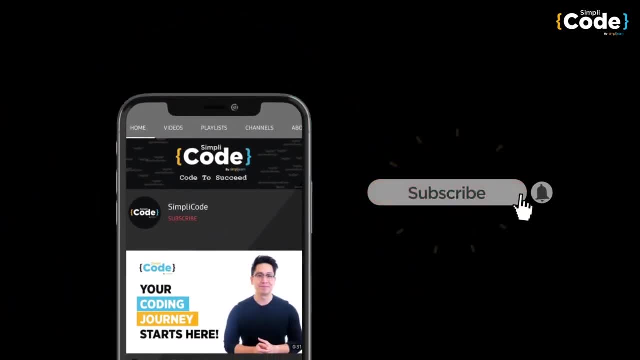 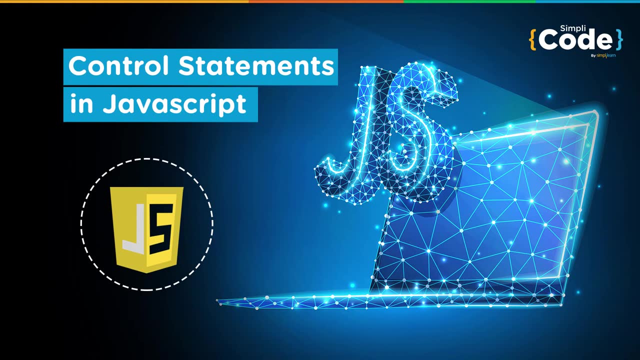 Hello everyone, and welcome to another video on JavaScript programming. My name is Kaushal and today I will take you through control statements in JavaScript. I will give you a brief introduction about how control statements work in JavaScript. So, without any further delay, let's get started. This video will be a small one because we'll 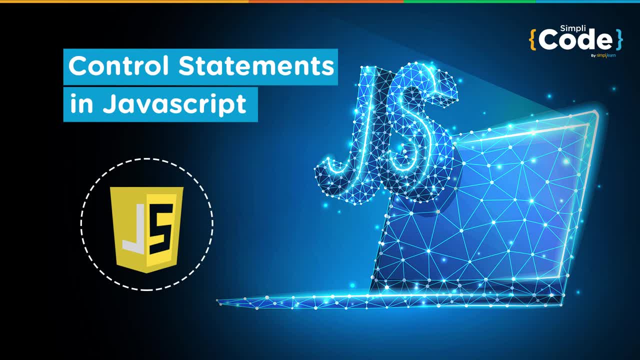 discuss each of these control statements in detail in separate videos, So the term control statement is pretty self-explanatory and straightforward, right? We came across JavaScript statements in previous videos. JavaScript statements are the instructions that tells the browser to perform specific actions. Control statements are also instructions. 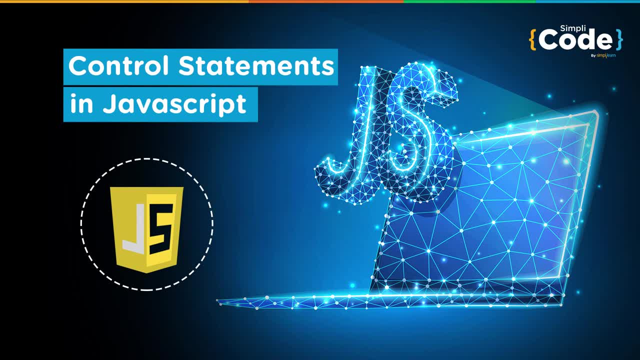 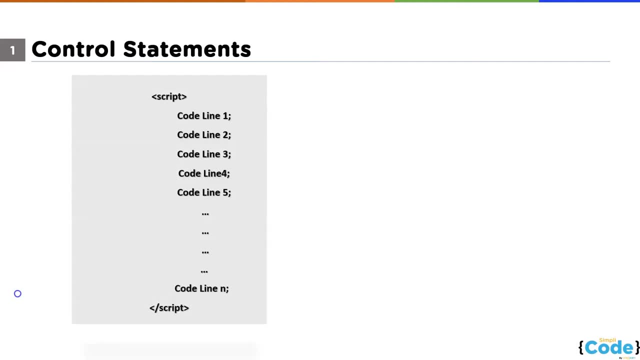 and they govern the flow of control in a program. So let's take a look at control statements with the help of an example. Let's suppose we have a piece of code that has n number of statements Here. let's say we have this code, and so the conventional workflow will be. it will first. 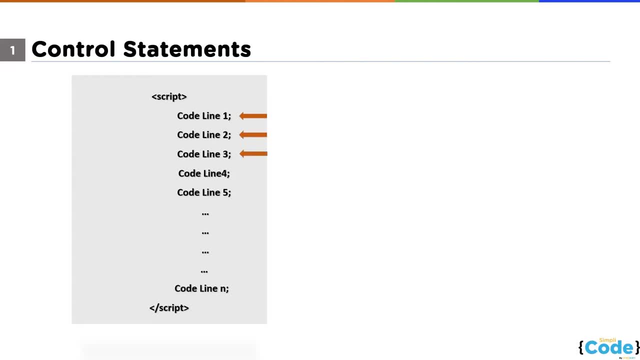 execute the first statement, then second, then third and so on till statement n, right? So this is the basic flow, right From statement one till statement n, and it will execute each statement in between. However, in real world, the scenario is: 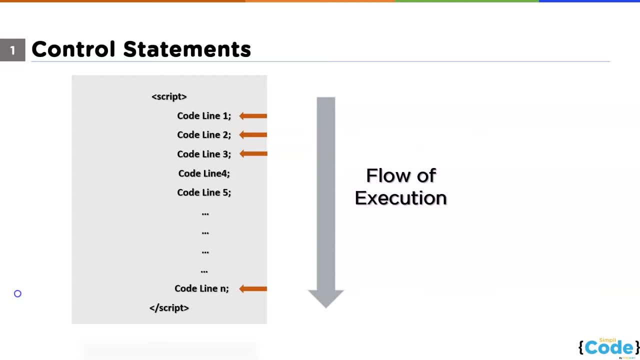 different, Like we don't write the code in same manner every time. For example, let's suppose you are in line 5 and you want to print this line 10 times. So what should you do? You can write this line 10 times, or you can copy paste it, right? Okay, let's forget about 10 times. Let's suppose 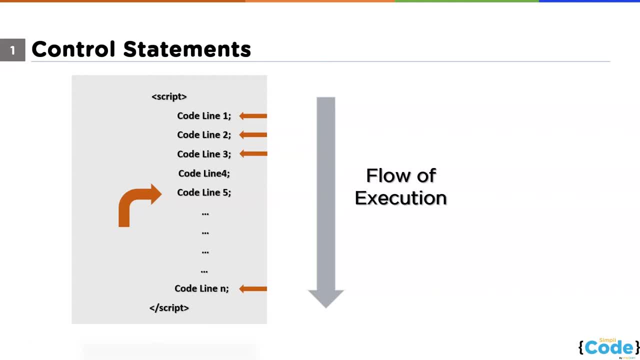 you have to use this code. or we can say: let's suppose you have to print this statement 100 times, Copy pasting it for 100 times, or writing this statement for 100 times. that's useless and unnecessary, right? So that's where control statements comes into the picture. We'll discuss. 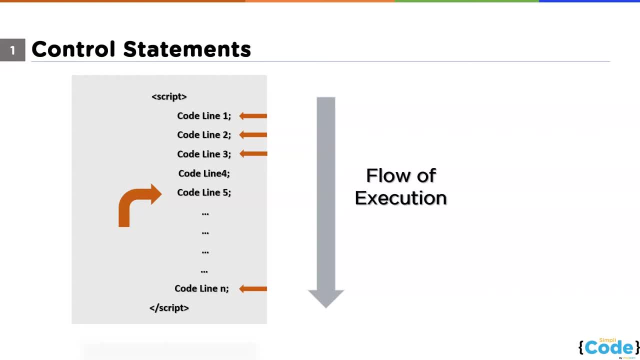 them in a while. Let's assume another situation. This time you want to make a choice based on certain conditions. You can use conditional operators, but then it has limitations. right To tackle this problem, we have control statements in JavaScript, So these are the very basic. reasons why we need control statements. Click Describes. If you color this detail, it will tell you about bound state in Java And by the next step we will have a facile way of displaying control states on JavaScript style. That's one of the simple things that you need. 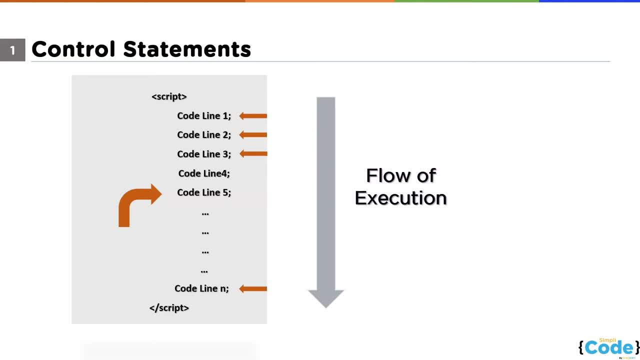 isn't it. You don't have engine. Is there a machine that makes this type of issues? You can't pass these. we need control statements for performing a certain activity, like if we want to perform a certain activity n number of times or if you want to make a certain decision making. 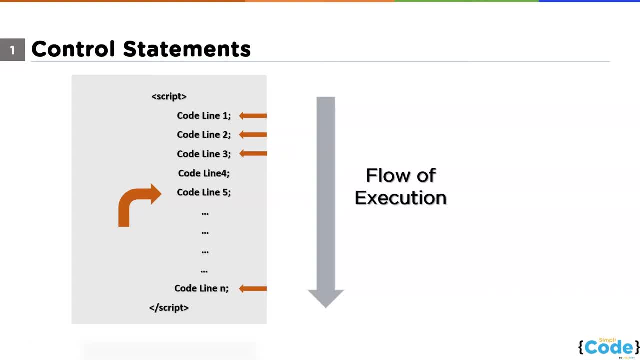 kind of scenarios in your program. that's where we need control statements in JavaScript. In JavaScript we have two different types of control statements, depending upon what action we are performing. So we have the conditional control statements and we have the iterative, or we can say looping. 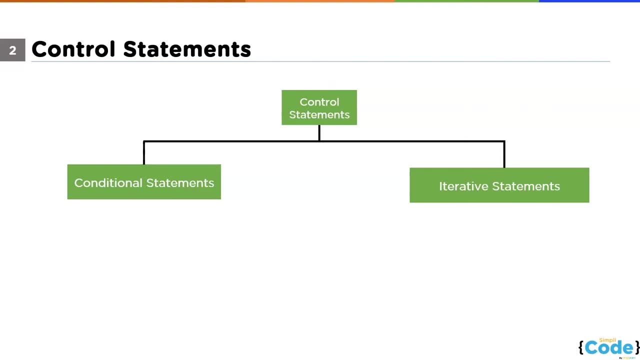 control statements. Talking about conditional statements, as the name suggests, we use conditional statements when we have to make decisions based on conditions, when we have two choices or when we can say when we have two different conditions and we want to make choices accordingly. So that's where we use conditional statements. 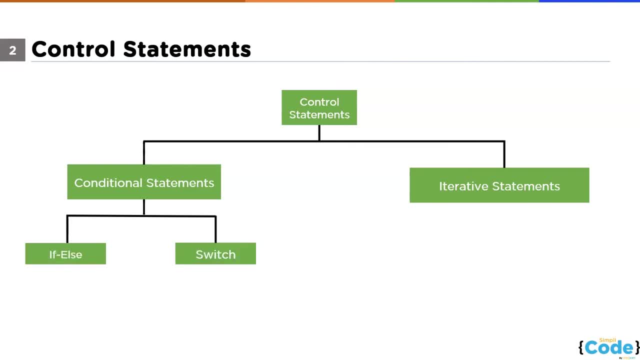 We have two different types of conditional statements: the if else statements and the switch case. Talking about the iterative statements, As the name suggests, if you want to perform any action more than once, or maybe n number of times, instead of writing them again and again, we use loops. 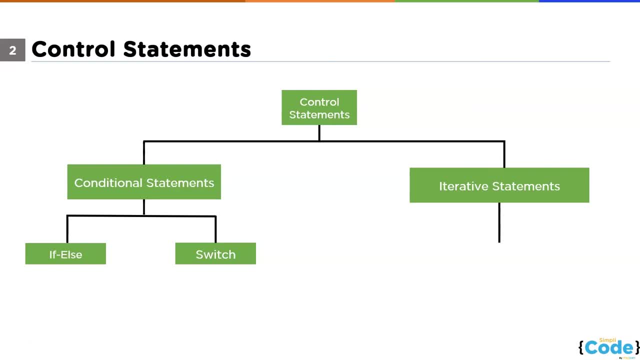 So loops are basically statements. we use loops to perform any activity n number of times with specific conditions. So in JavaScript we have four different type of loops. we have for loop, while loop, do while loop and for in loop. So the for loop, while loop and for in loop. 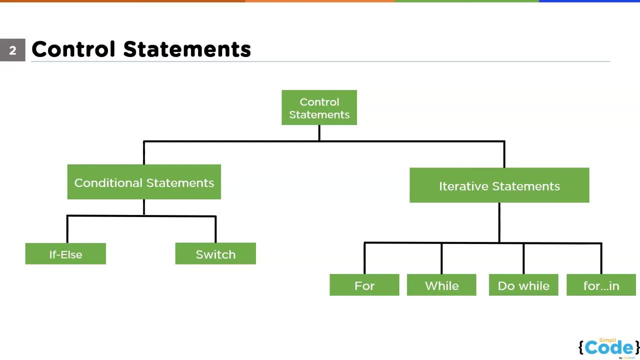 So the for loop, while loop and for in loop. So the for loop, while loop and do while loop. You might have heard about them earlier because they are also present in other programming languages. but this for in loop. this is a new type of loop present in JavaScript. 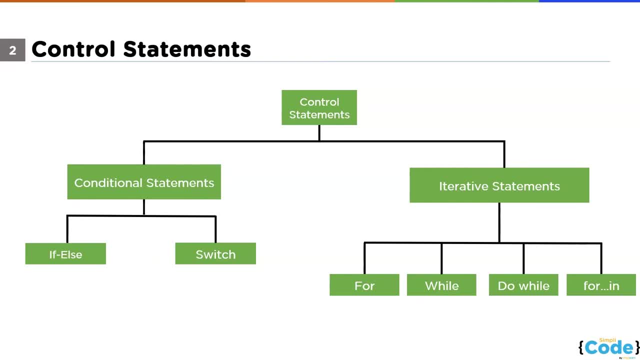 We use for in loop with objects. we will go through objects in upcoming videos and, of course, we will be looking at each of these control statements in detail. we will have a particular video for each of these topic. Now let me introduce to you The break and the continue statement.